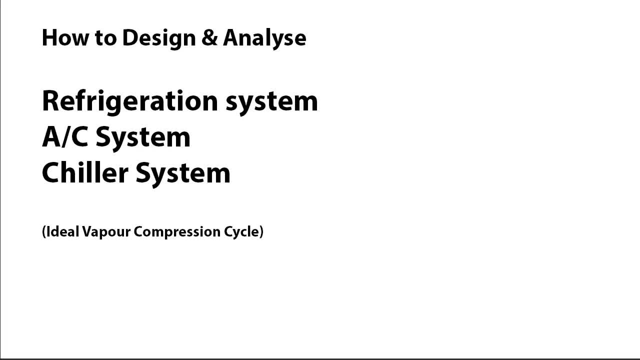 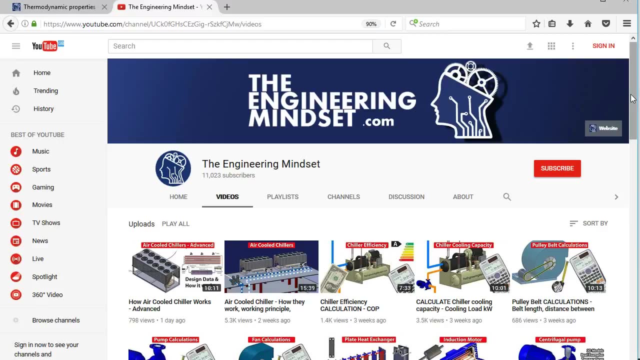 they're just a slightly different scale of size. But also remember that this is going to be for an ideal vapor compression cycle, So the performance of this would be slightly different to the real world scenario. So this is the theoretical version of it. Now, if you're a new viewer to the channel, then I'd highly recommend you check out our 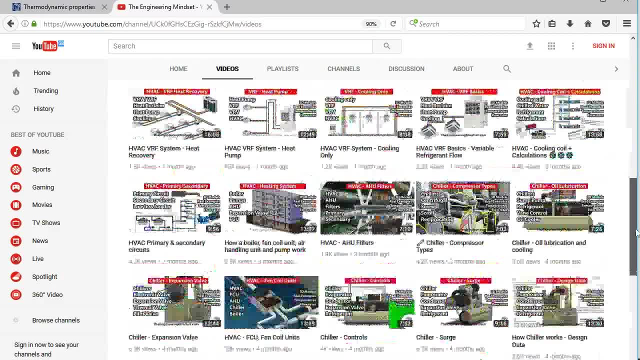 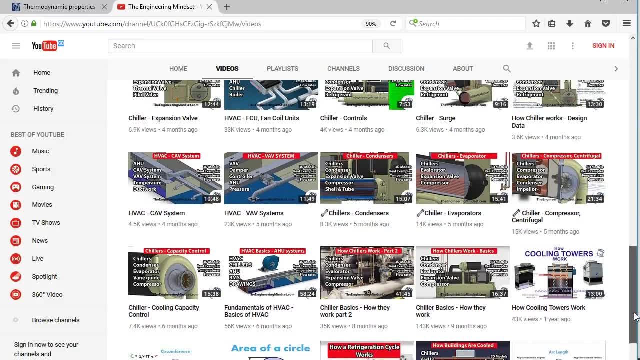 other videos, as we cover everything to do with HVAC and buildings. Some of the ones you'll probably be interested in are the basics of the refrigeration cycle and also the chiller basics, how they work, as well as fundamentals of HVAC. Thanks for watching. 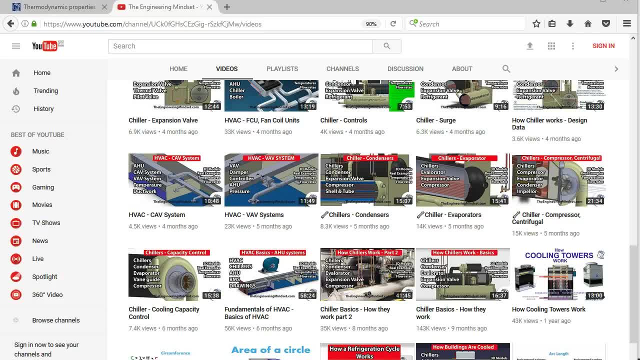 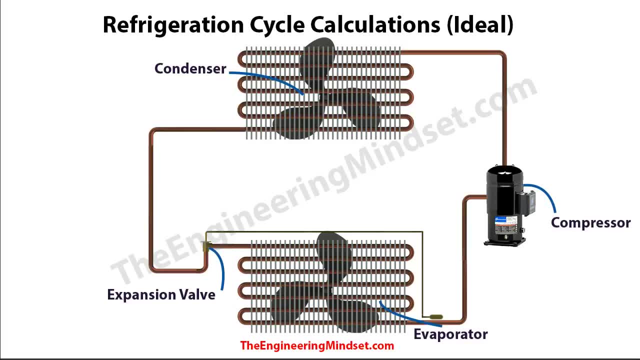 So if you haven't checked those videos out, I highly recommend you go and do so. Anyway, straight into the video. So here we've got our basic refrigeration cycle. You probably know what all these components are by now, but I'll just label them up. So we've got. 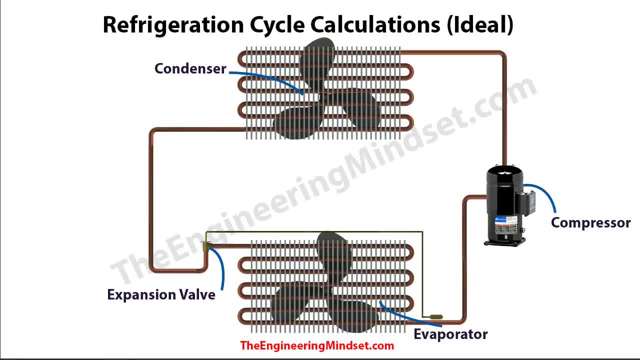 the compressor, then the condenser, the expansion valve and also the evaporator. The compressor compresses the refrigerant and pushes that around the system. The condenser rejects the heat, the unwanted heat, from the system. The expansion valve expands the refrigerant and 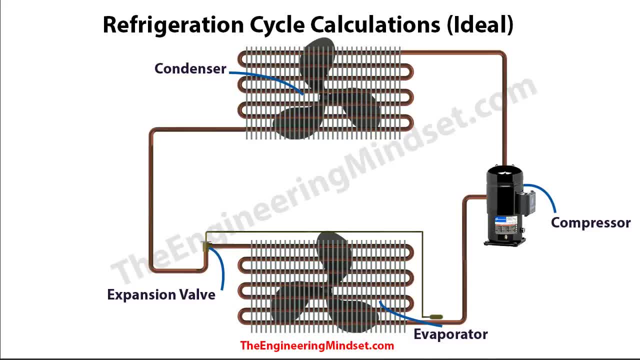 Crimeank techn Roget. And the evaporator absorbs the unwanted heat that's coming in from the building. It's also produces the cooling which goes out to the building. Now to design and analyze a refrigeration system or cycle, then we want to know what the thermodynamic 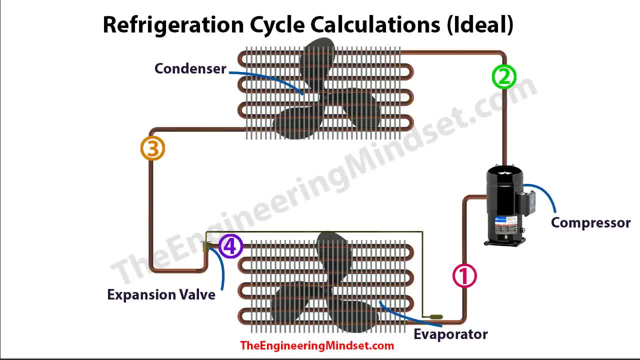 properties of the refrigerant is going to be at four key components, Being point one here or stage one between the evaporator and the compressor, Then stage two, which is what state is it in when it leaves the compressor, What stage of how the model is going to be. 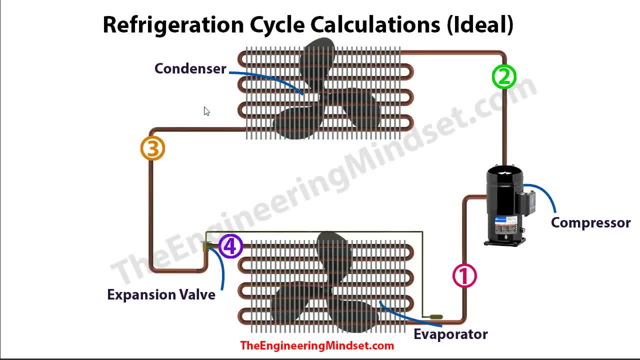 compressor. State 3 is going to be what the state is of the refrigerant when it leaves the condenser before it enters into the expansion valve. and state 4 is going to be the condition of the refrigerant just after the expansion valve, before it enters into the evaporator. So the four main. 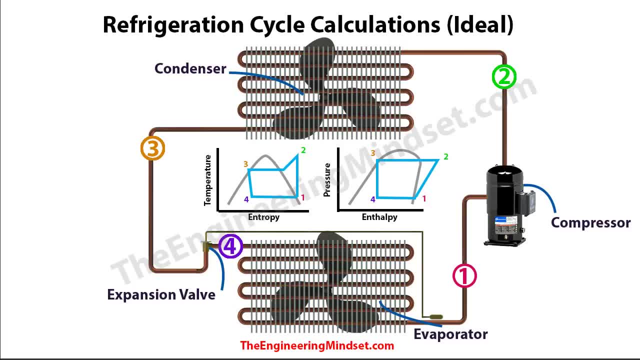 things we want to know about the refrigerant is going to be its temperature, its entropy, its pressure and its enthalpy at all four of these points. Now, if you haven't seen these charts before, then this is the saturation line, this gray line here. so anything to the left of 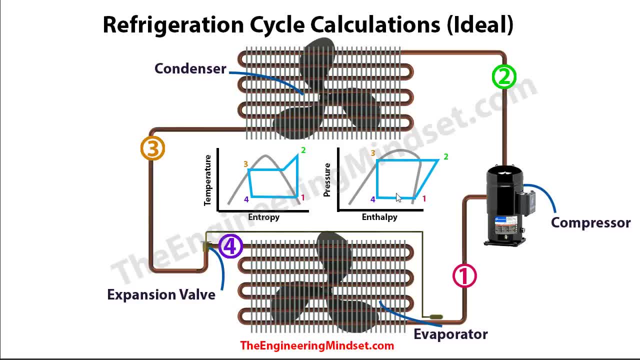 this is where the refrigerant is liquid. Any point where it's in between, this is where it's going to be some kind of vapor, liquid mixture, and anything to the right hand side of that is where it's going to be a superheated vapor. So if the line is touching on here, 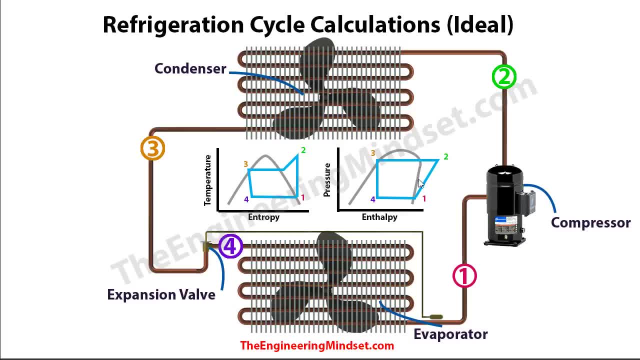 then that's going to be a saturated liquid and if it's on this line here, that's going to be a saturated vapor. So from these graphs we can see that point 1 here is going to be a low temperature. it's also going to be a low pressure and it's going to be a saturated vapor. So we'll start to plot these as: 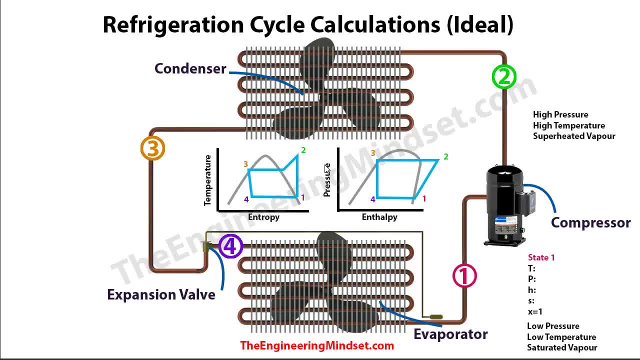 we go around State 2, we can see that it's going to be a much higher pressure, so it's gonna be a high pressure there. it's also a high temperature and it's in the superheated region, so it's a superheated vapor. Now at point 3 over. 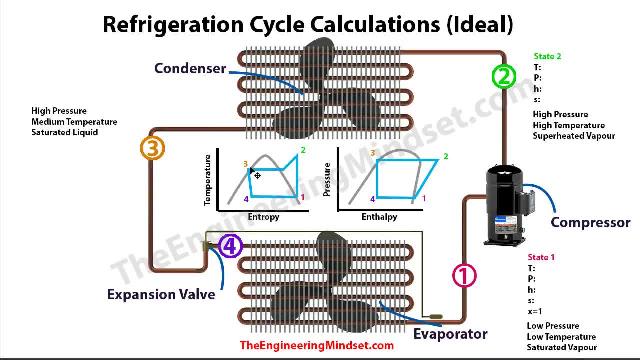 here we can see that it's still a high pressure. it has reduced slightly in temperature, so it's a medium temperature, and it is also on the saturated liquid line, so it's going to be a saturated liquid. and we can also see that point 4 just after the expansion valve, when that refrigerant has all been. 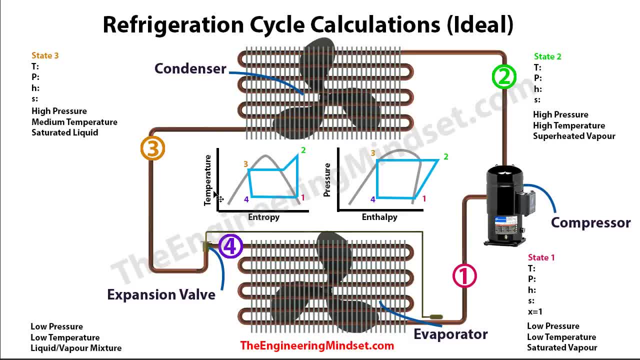 expanded, we can see that that's going to be a much lower pressure and temperature. so it's a low pressure, low temperature and it's in between the dome. so it's going to be a liquid vapor mixture. Now just to clarify what some of these acronyms are, as I've put them around. so T is going to 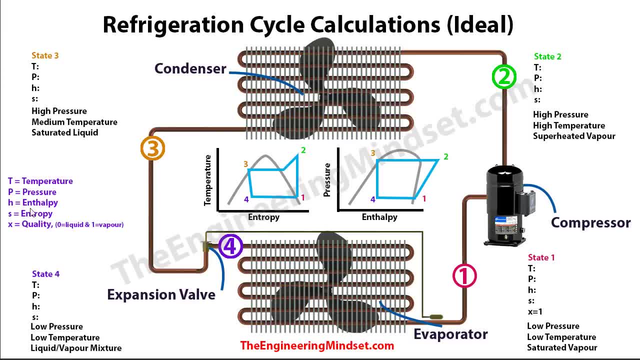 be for temperature, P is going to be for pressure, H is going to be for enthalpy, S is going to be for entropy and X will be the quality of the refrigerant. So you can see that I've put zero if it's a liquid and a one if it's a vapor, so that 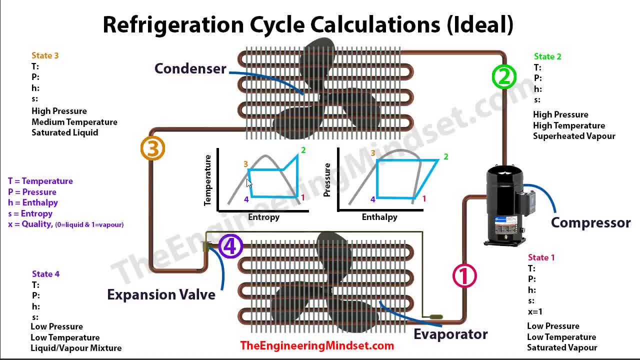 is just to work out how far between being a liquid and a vapor the refrigerant is when it's in the dome there, and we'll see why that's important shortly. But you can see for example just here: X equals 1, so that lets you know that it is a saturated vapor. it's right on the line there Now. 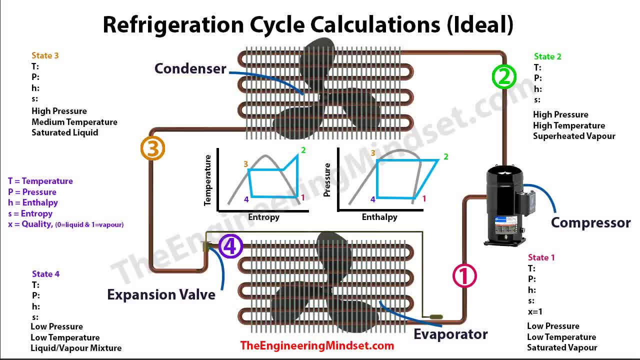 there's lots of ways that you can start to design one of these systems. probably knowing the cooling load that you want to achieve would be a very good point to start with. So how much cooling capacity does your evaporator need? But in this video, we're just going to show you how much cooling capacity does your evaporator need, But in this video, we're just 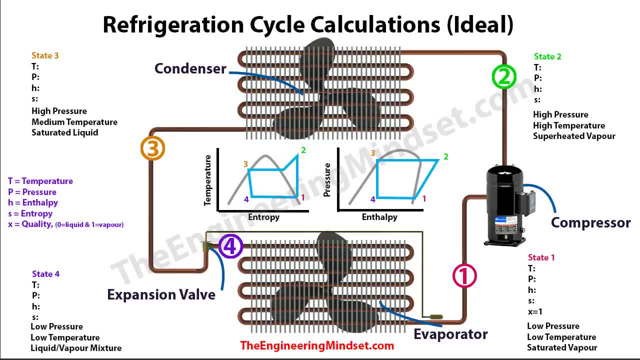 going to start from scratch, and really all you need to do is watch this video, learn how we calculate things and how we look the properties up, and then you can tweak these to your own version to design the system that you need. So we're going to start with the compressor. So I've got a compressor that's able to. 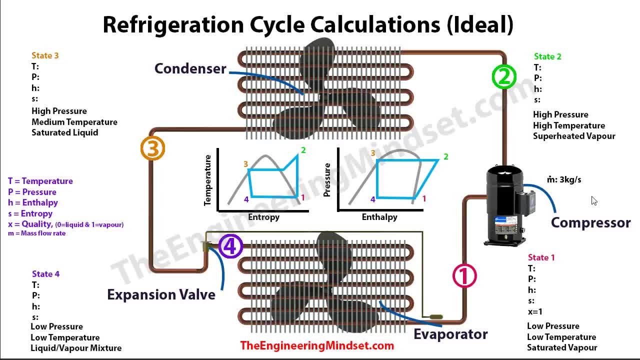 provide or push seven kilograms a second of refrigerant around the system. I've just added the M dot over here as the acronym, so you know what that is. but M dot just means the mass flow rate. The dot represents the rate Now from the. 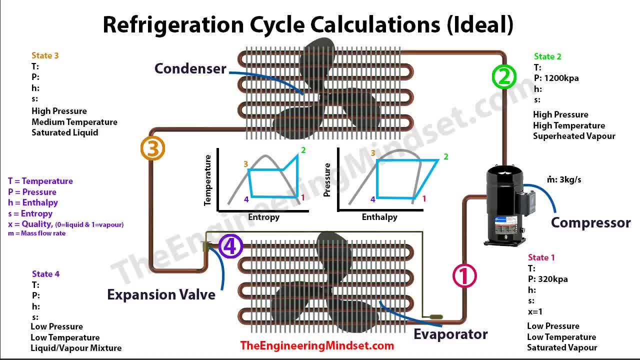 manufacturer's data. this chiller is able to produce 1200 kPa of pressure, and it also needs a suction pressure of 320 kPa. So we just add those values in there, And now we'll start to fill in some of the data that's missing here. So we know. 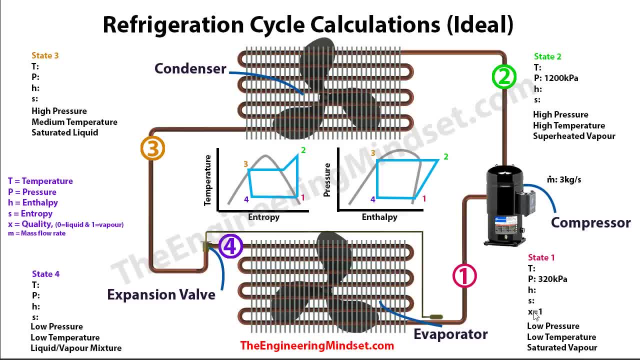 that the pressure is 320 kPa and that it is a saturated vapor on the on the saturation line, And then we just need to look up what the values of these are going to be on the thermodynamic properties of refrigerant R134A or whichever refrigerant you're using. In fact, I'll just add that in there. 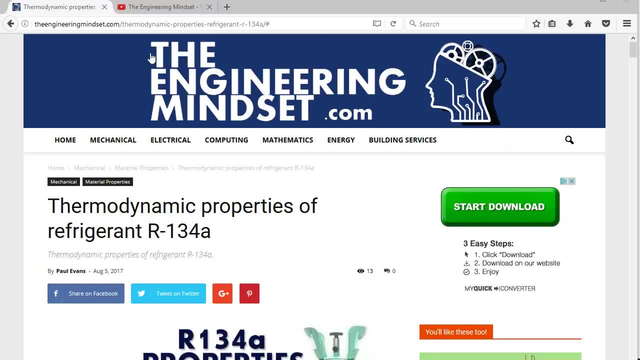 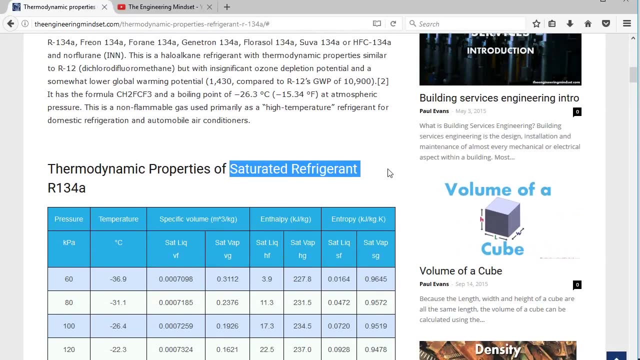 so we know which refrigerant we're using. So if you check out our website, TheEngineeringMindsetcom, and specifically if you go to this page here- thermodynamic properties of refrigerant R134A- and we then scroll down and we'll see, we want to find this is the saturated refrigerant tables, so we want 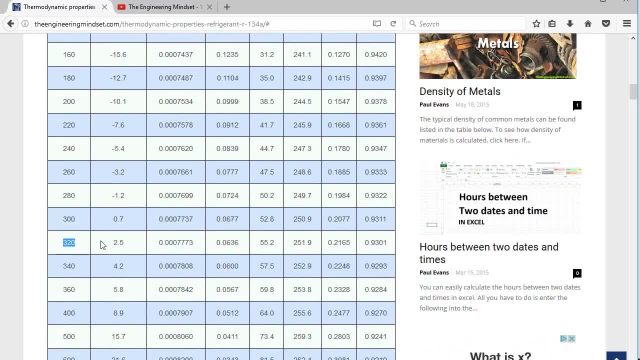 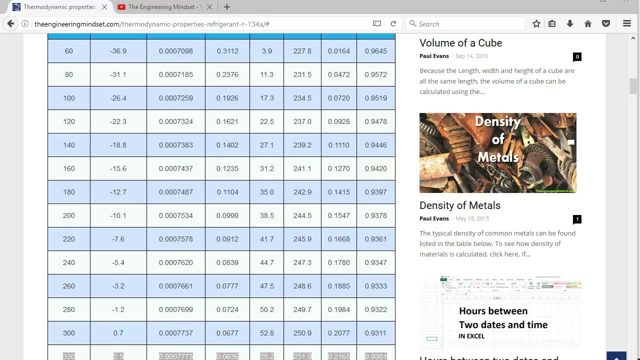 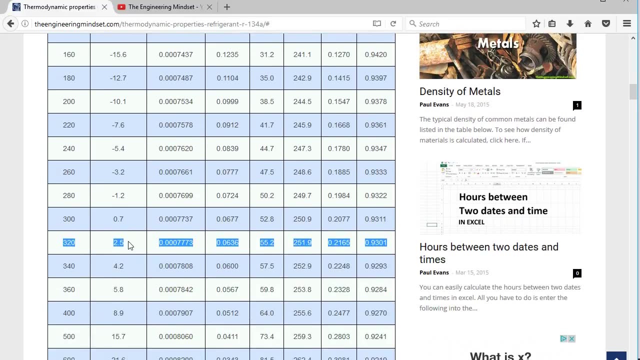 to find 320 kPa, which is this line here, And we want to know what the temperature, enthalpy and entropy are at this point. So on this line here, just change that a little bit. we can scroll to the top and see that this column is the temperature. 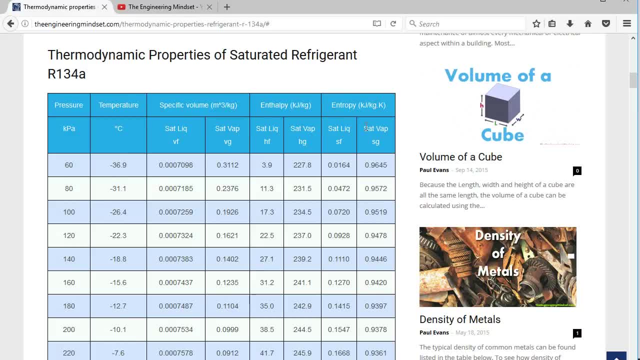 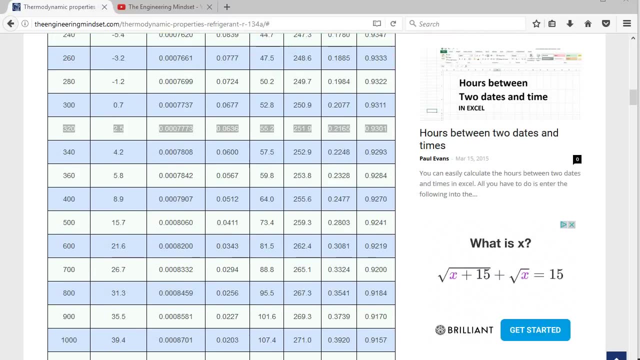 this is the enthalpy and this is the entropy. Obviously, we're on the saturated vapor line, so we got the saturated vapor of that one and saturated vapor line for the enthalpy as well. So we're going to want this column, this column and this column. So we want this value here, this. 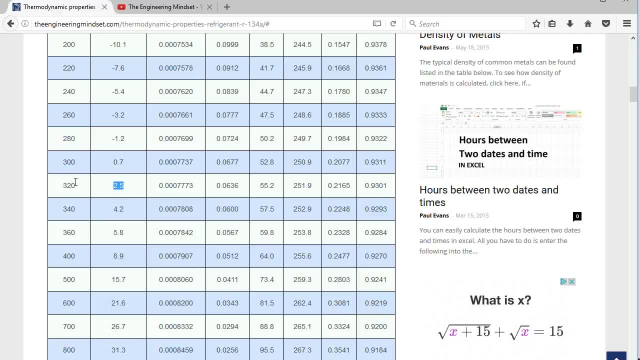 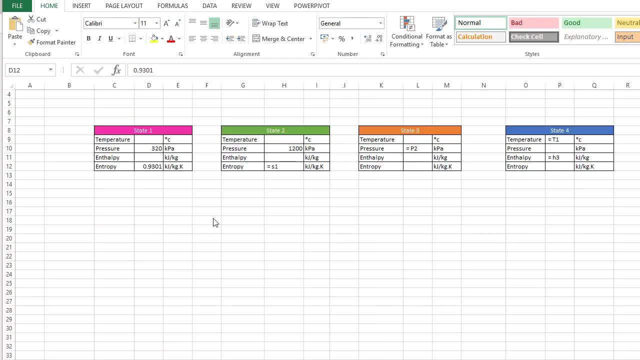 value here and this value here. So let's just zoom out and copy that over. So So we'll take this cell here and we'll just paste that into Excel. You don't have to do this, You could write it by hand as well. 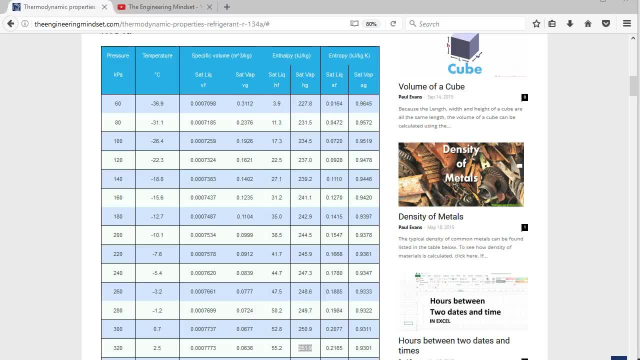 I'm just using Excel. It's a bit easier and quicker. Then we'll take the enthalpy of the saturation saturated level and just paste that in as well. Then we just take the temperature and we paste that one in as well, And I'll just update that front sheet there. 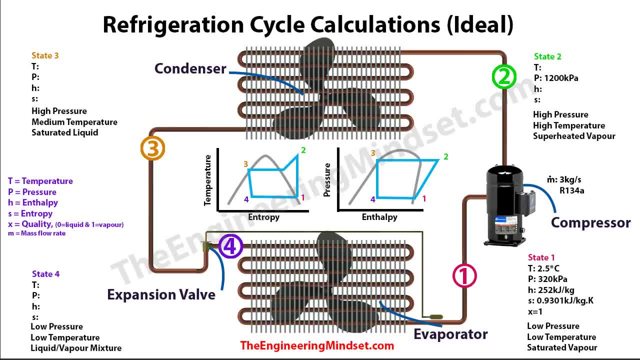 And now we'll have a look to find what the properties of the refrigerant are at state two. Now, to look at the properties of the refrigerant up on the tables, we need to know two points to reference that. So at the moment we just know what the pressure is and that we know it's a 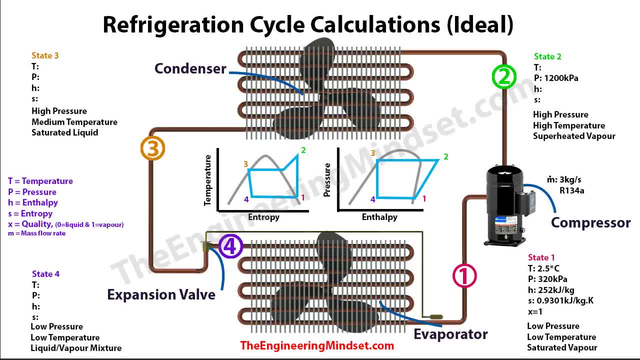 superheated vapor, but because we're doing this as an ideal cycle. that means it's the compressor is isentropic and that means that the entropy at state two equals that at state one. So I'll just drop that figure in there. 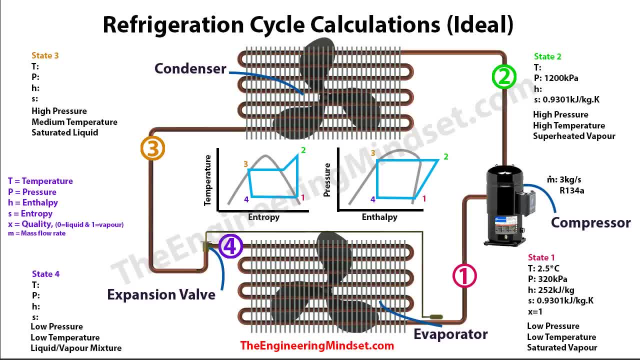 That's come from the left. And now we can look in the superheated vapor tables to find the enthalpy and the temperature given the pressure and the entropy. So if we come back to the website and we scroll down through the properties of the 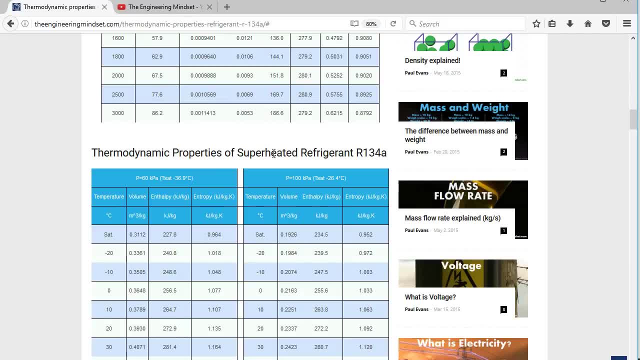 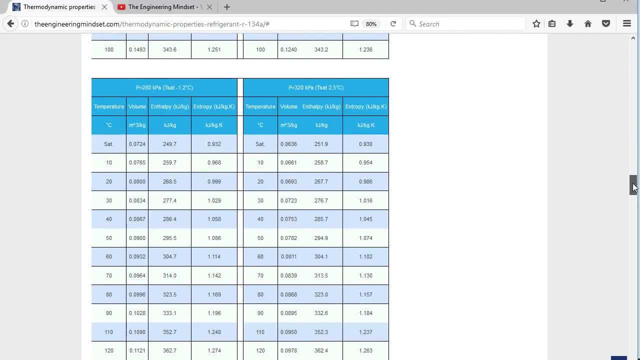 refrigerant R134A, and you'll see we'll come to the superheated refrigerant. So we're looking for 1200 kPa. So these are too low. We'll come down a bit more, a bit more. We've got one for all of these. 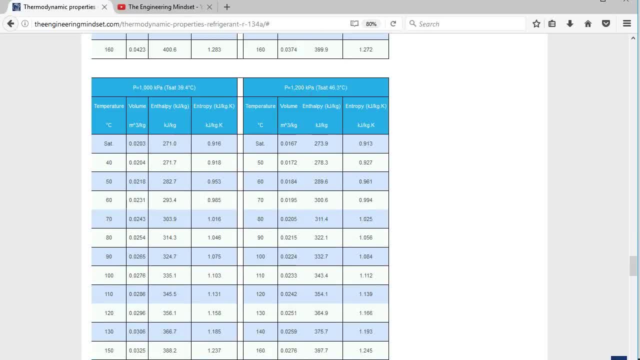 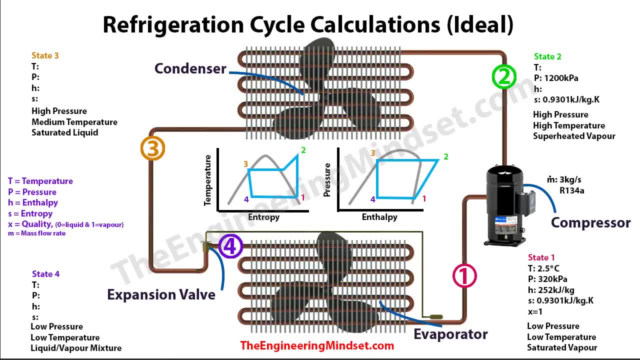 All of them over here. there we go: 1200 kPa Now. the entropy we're looking for is 0.9301 kilojoules per kilogram per Kelvin, But looking down this list you can see it's not quite there. 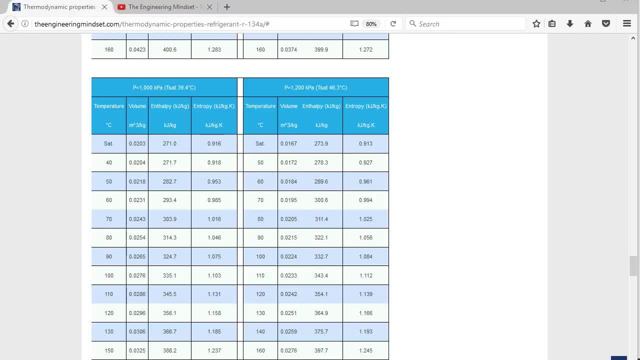 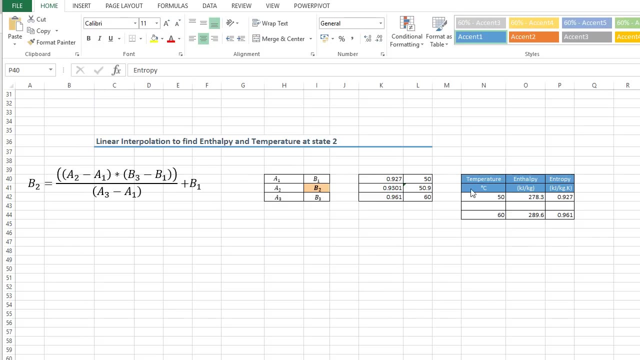 It's actually in between these two here, but that's okay, We'll just have to use some linear interpolation to find that value. So if we highlight and then copy and paste these values here and just drop them in Excel, and we'll just drop the values in there. 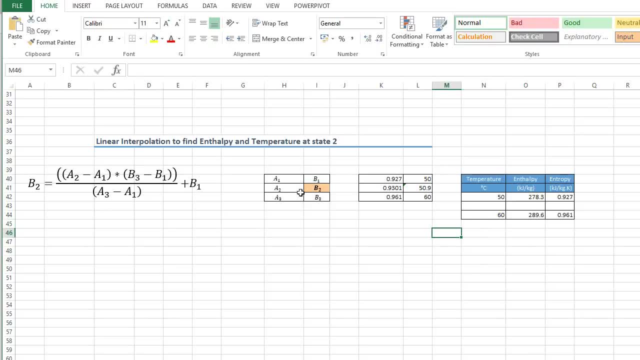 Now we can use this formula here to calculate what that's going to be. So we know these three A's and we also know the B1 and B3, but we don't know B2.. And what I mean by that is we know at 50 degrees what the entropy is going to be. 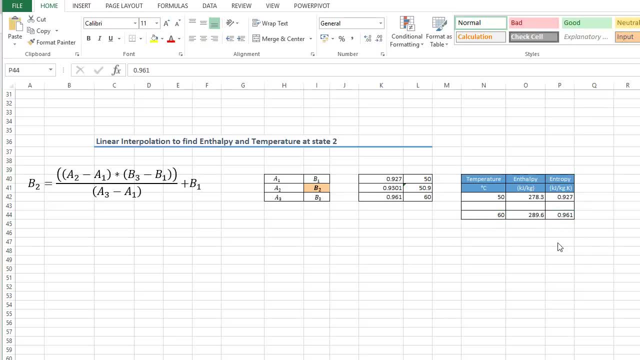 and at 60 degrees, what the entropy is going to be. but we want to know what the enthalpy and entropy is going to be going to be at naught point nine three zero one. so therefore, these will be our A's and these will be our B's. now I've already pre-made the calculator for this. 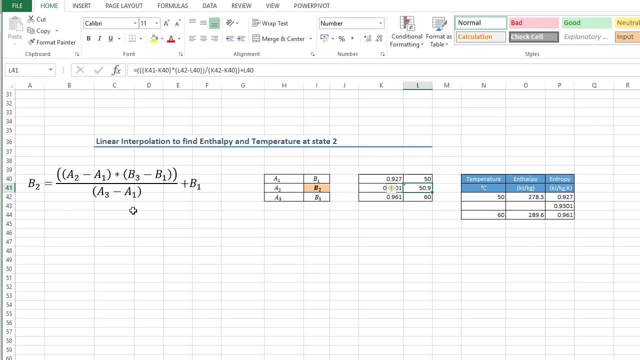 so I'll just show you the formula there. it's just this formula here, but in the Excel version, so we'll just drop the numbers in there. so we'll take the 50 degrees Celsius, drop that in there, six degrees onto here, and then we'll take. 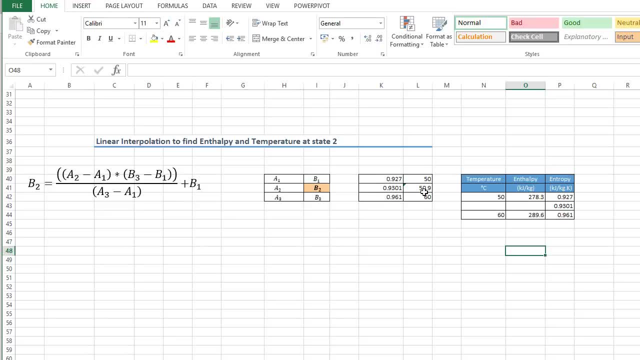 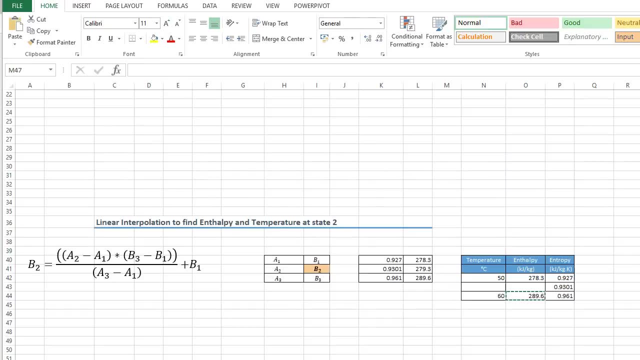 these three numbers there and we'll drop them in and that will give us the temperature there, which is now 50.9 degrees Celsius. so that's at the table, and then we can find out what the enthalpy is by doing exactly the same, just moving this enthalpy over and this enthalpy over, using that same formula. 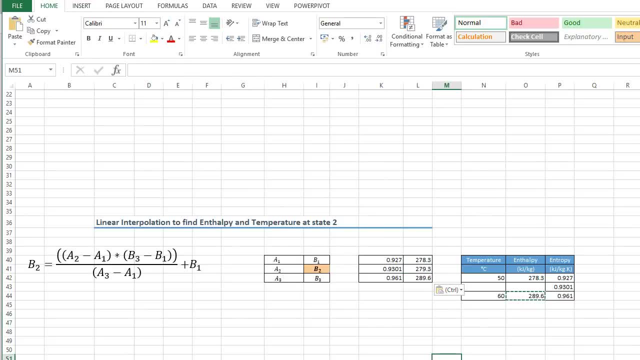 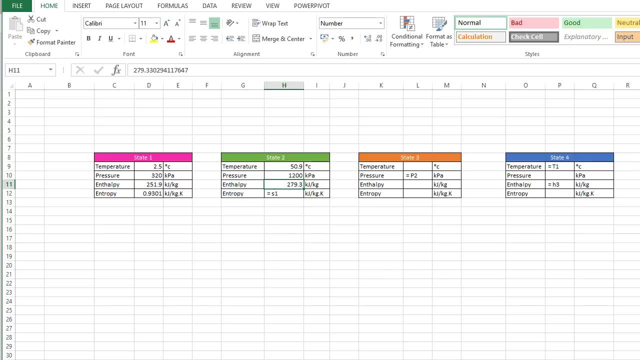 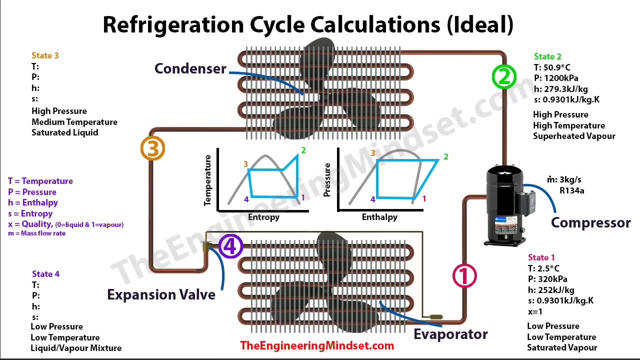 and that will give us what the enthalpy is at the correct entropy that we need. so we'll just copy and paste that over into our table. Obviously, we know that the entropy was the same as this cell here and we just update the overall table there. Now, as this is an ideal system, there is no. 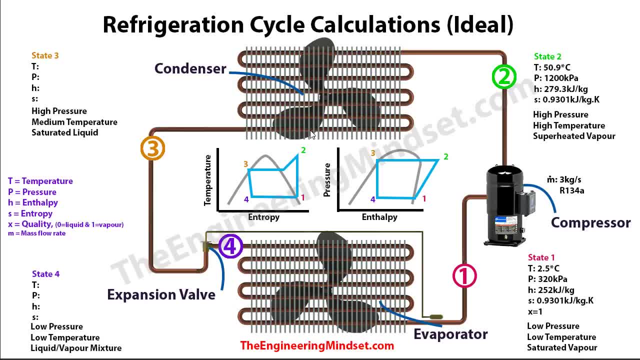 resistance in there. so there'll be no pressure drop in the real world. obviously there will be some pressure drop, but for this ideal scenario then we're just going to take the pressure from here and we'll assume that is the pressure at state 3.. So now we've got the pressure and we know that it is a. 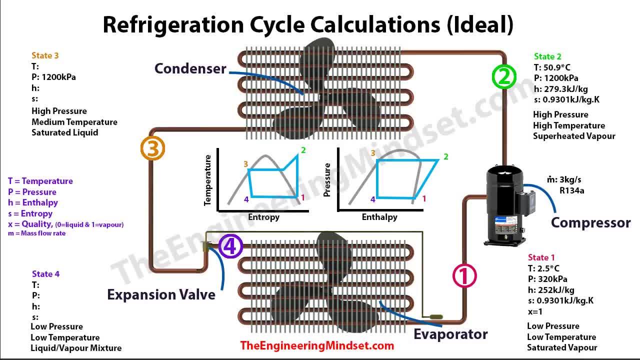 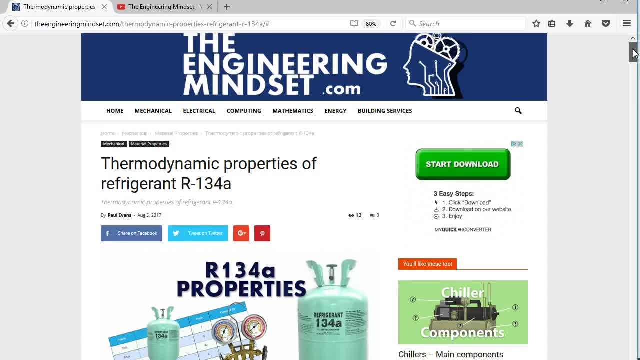 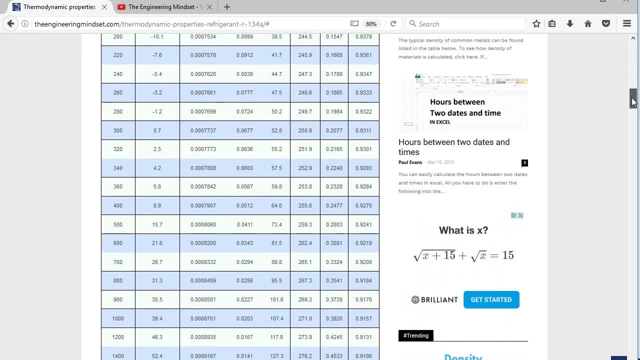 saturated liquid and that means we can use the saturated liquid tables to find out the temperature, enthalpy and entropy. So, coming back to the site and the properties tables, we'll just scroll down. we've got the saturated refrigerant tables there and we're looking for 1200 kPa. there's the pressure on this line. 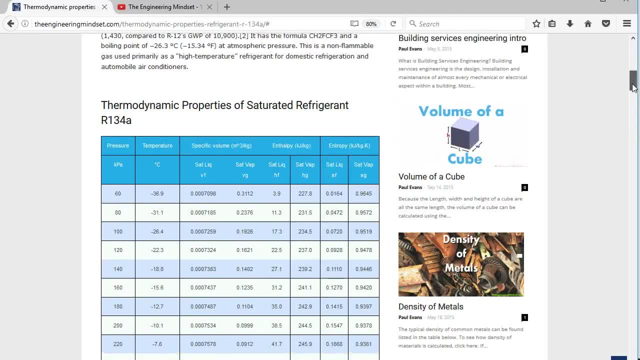 here and we know that it's a saturated liquid, so we want the saturated liquid column. so the entropy: we want this one here. the enthalpy: we want this column here and obviously we've got the temperature over there, so we just scroll down and so we want this value here and 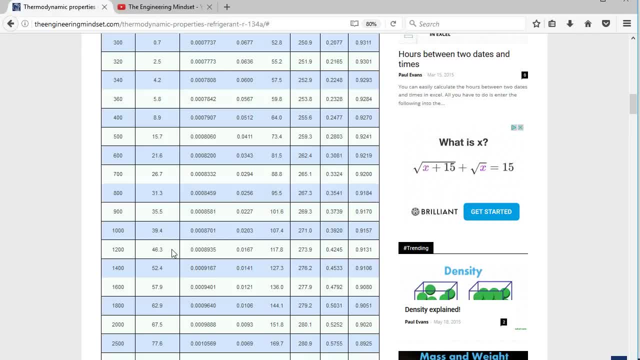 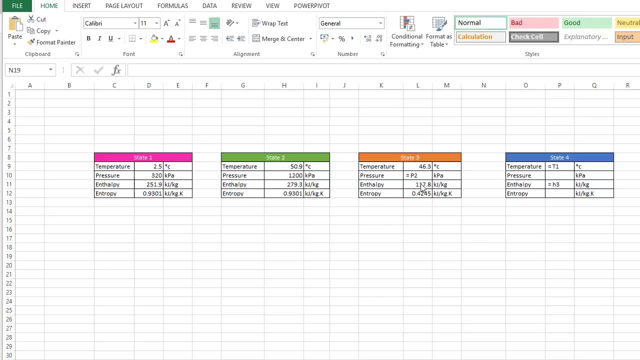 this value here, as well as this temperature here. so we'll just copy and paste those into the excel sheet. there you go. we just drop these in there, and we also know that this pressure is going to be the same as P2, and I'll also just 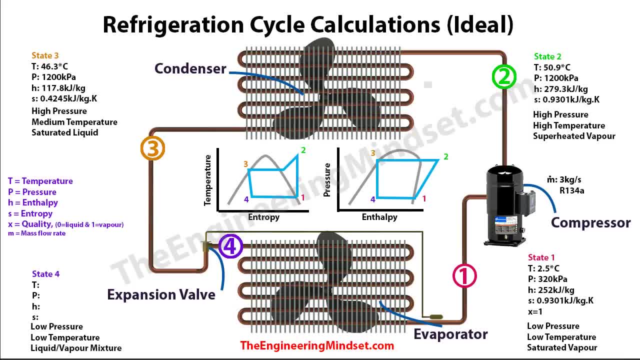 update the front sheet there. and now we need to know what the properties of the refrigerant are going to be at state 4, and this is slightly more tricky because obviously it's in between the vapor dome. so it's part liquid, part vapor, and we're. 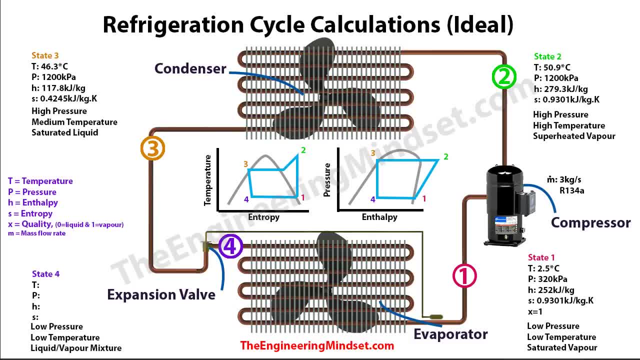 not sure exactly yet how much vapor or liquid it is, but that's okay because we can just work it out. so we know here that the temperature is going to be the same as the pressure at state 4, and we know that the pressure is going to be. 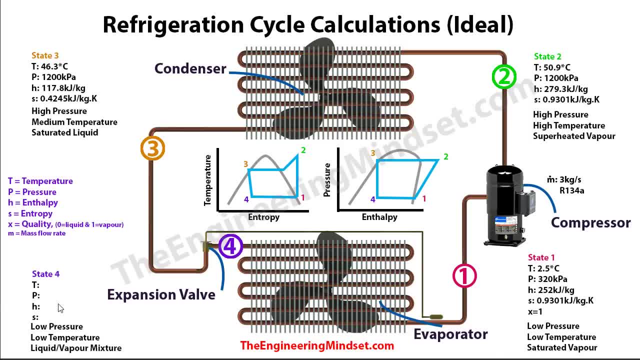 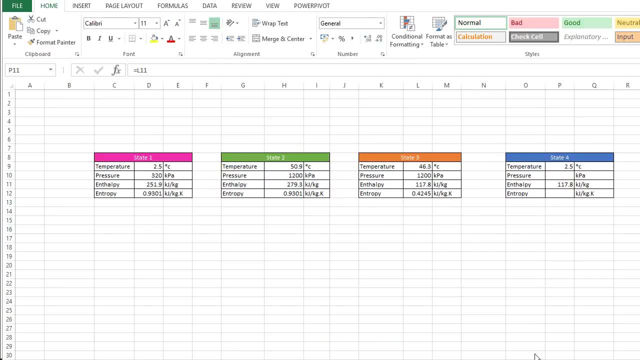 as 0.1 and that the enthalpy will remain constant through the expansion valve. so that means, we can use the enthalpy from state 3, so if we drop those figures in there and also drop them into our excel sheet at state 4, now we also know what. 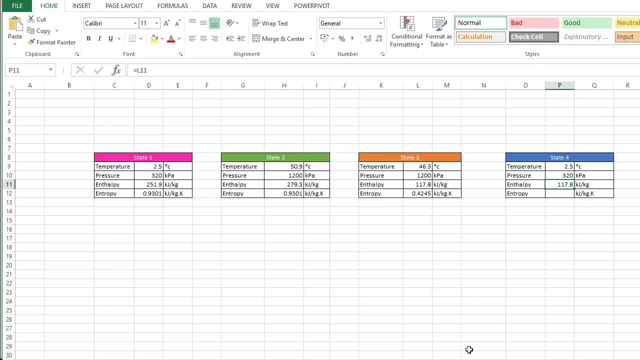 the pressure is, because that is going to be equal to state 1 and that means we only need to find out what the entropy is. and the way we do that first is by finding the quality of the refrigerant. so how much or what part liquid or vapor do we have? and for that we come back to 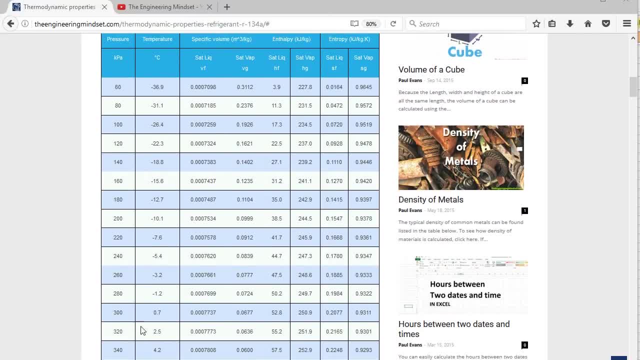 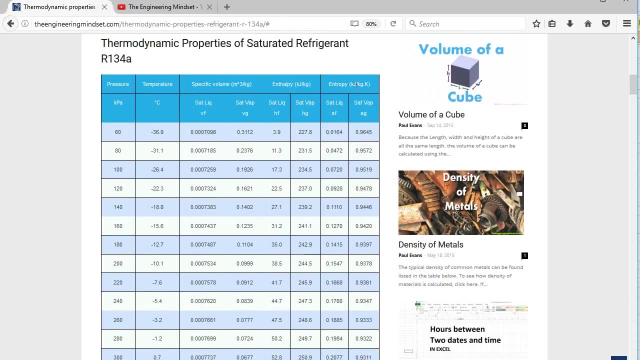 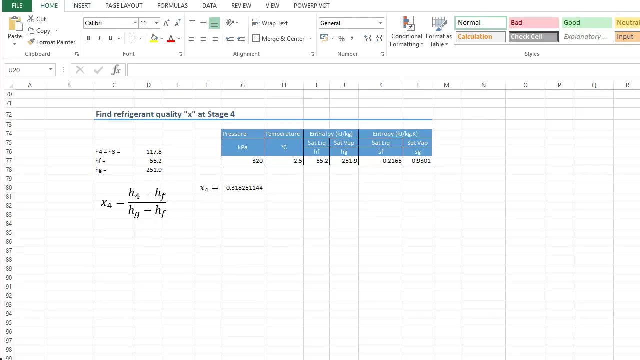 the saturated refrigerant tables and we scroll down until we find the 320 kPa line. and then we want to copy and paste all these values, or just the entropy, enthalpy, temperature and pressure, and we want to take those for both the saturated liquid and vapors. and now to find the quality of the refrigerant. we're going to use this formula here. 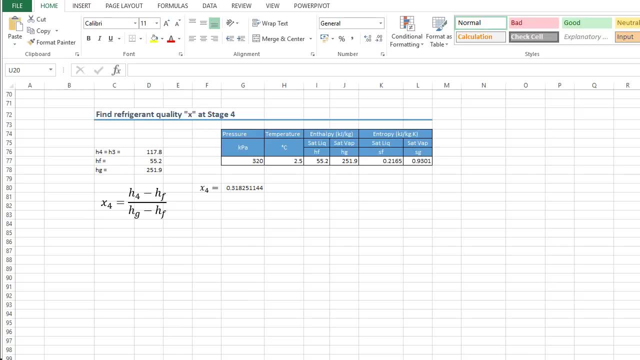 so x being the quality and h representing the enthalpy. so we already have the value of h4, because that was a equal to the enthalpy at point or state three. and we also know what hf and hg are because we've got them here on the table. so hf is the saturated liquid and hg is the saturated 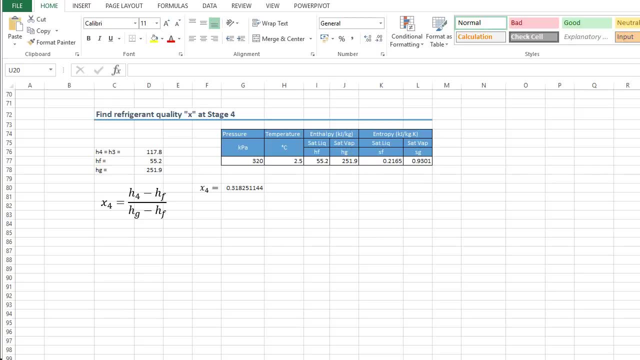 vapor value, and we took these from the charts on the website, so now we'll just use this formula here, but i've put them into this cell here. you can see the formula up here is exactly the same as this one here, and when you drop these numbers out you'll see that this comes out as a decimal. 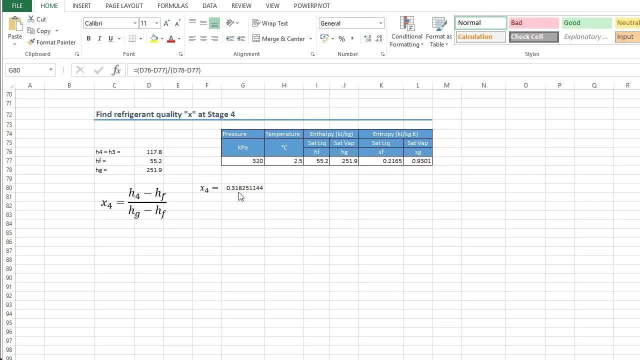 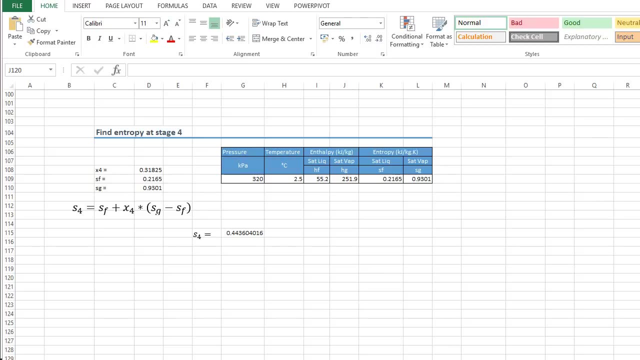 because it's a ratio, and so it's 31 of almost 32 percent. so now we use that quality that we've calculated there to work out what the entropy is going to be at state four, and we do that using this formula here. so we've just worked out what the quality is. 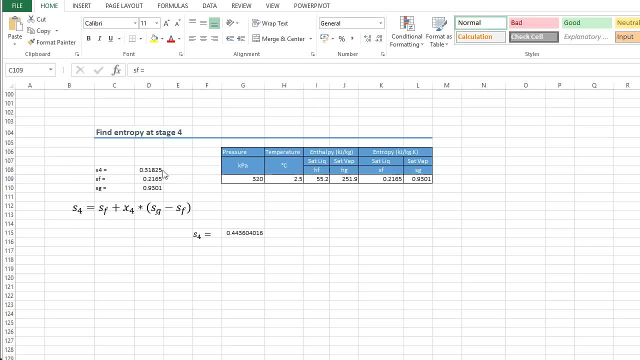 at state four. we know what sf and sg are going to be because we've taken them also from the tables and you can see sf is the saturated liquid and sg is the saturated vapor for entropy. sorry, so if we use this formula here, just this one here. 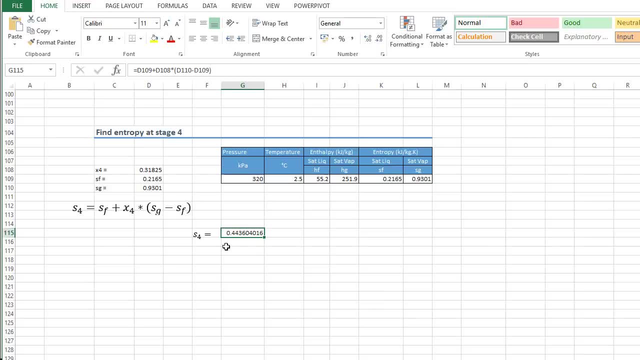 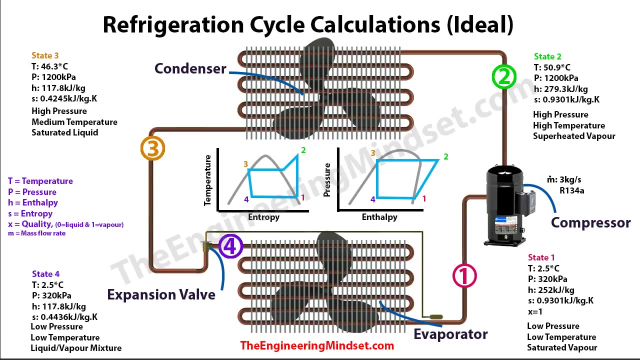 exactly the same there, just in the excel version, and we'll see that s4 drops out at 0.4436 kilojoules per kilogram per kelvin. so that's all the properties of the refrigerant worked out, but we still got some more calculations to do, so let's work out the amount of work done by the 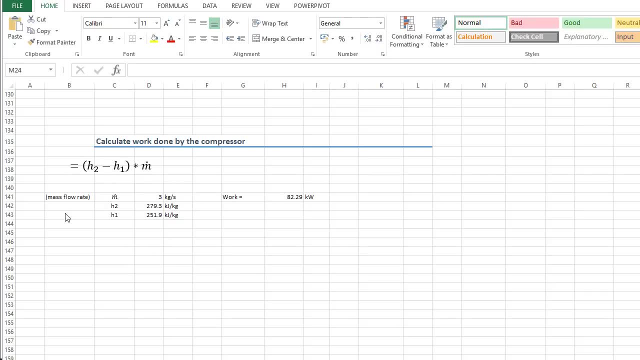 compressor. so we can do that using this formula here. so we've got the enthalpy of state two and state one, and we've got the enthalpy of state two and state one, and we've got the enthalpy of state one and the mass flow rate of the refrigerant. so how much refrigerant is the compressor? 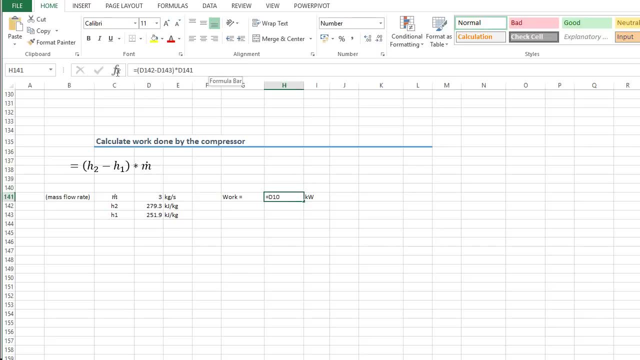 pushing around and we can use this formula up here which is using these cells to work out it's the compressor is doing 82.29 kilowatts of work on the system and we can also work out how much cooling or the cooling load on the evaporator by using this formula here. 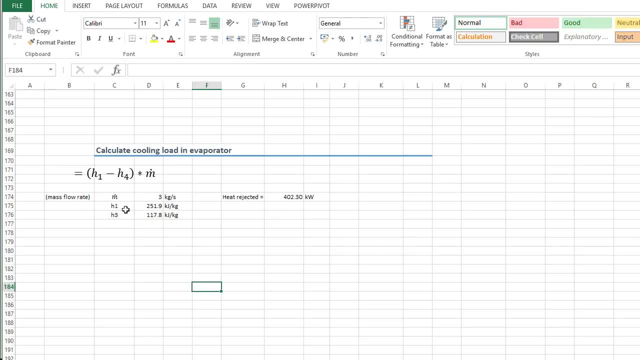 and it's almost exactly the same formula. we're just using the enthalpy from point one and the enthalpy from point three and we'll use this formula here to work out that it is providing 402 kilowatts of cooling. and we also want to know or calculate what is the heat rejection. 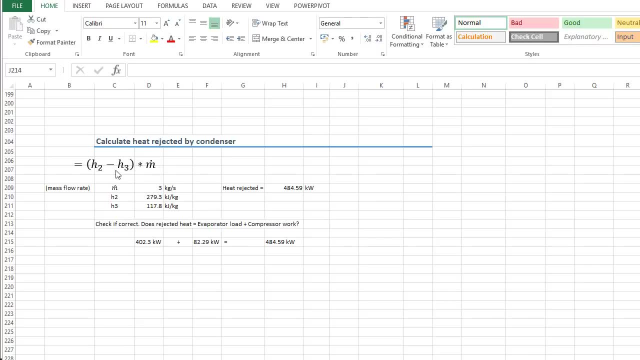 by the condenser. we can work that out using this formula here- again very simple and similar formula- and just using this formula here and that we can see it's 480.485 kilowatts. now you notice that that is higher than the provided and that's because we've got to get rid of the heat produced by the. 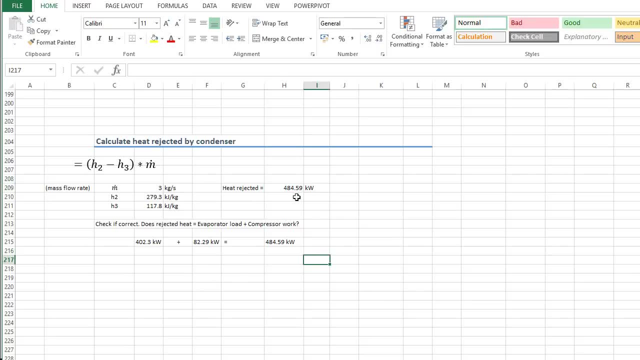 compressor as well, so you can add these together to to check if your figures are correct. so if you added the cooling load plus the work done by the compressor, you should equal the heat rejected by the condenser. if they don't equal, then you've done something wrong and you need to go back and just have a. 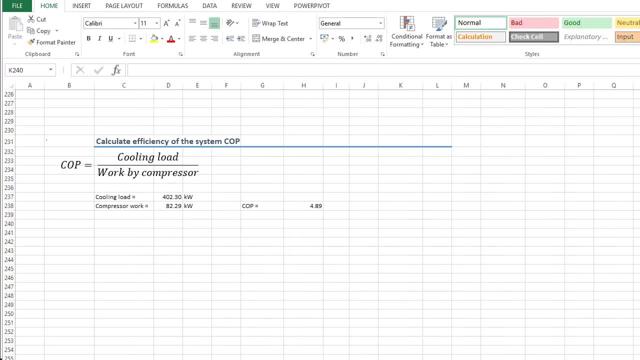 look through some of your figures and then we can calculate the efficiency of the system or the coefficient of performance, using this formula here, which is just the cooling load divided by the work done by the compressor. and we can use this formula here: very simple, just the division, the ratio, and that. 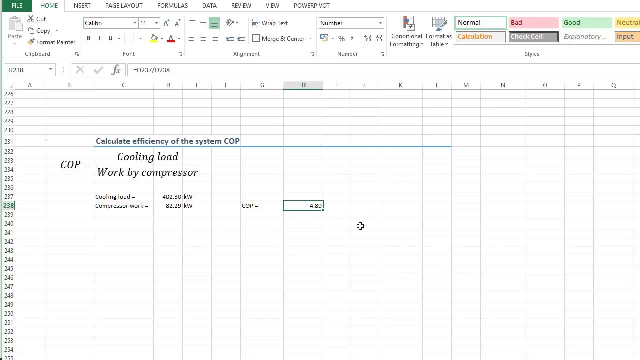 will work out that this system we've just looked at here is producing, or has, a coefficient of performance of four point eight nine. so for every kilowatt of electricity you put in, you'll get four point eight nine kilowatts of cooling, and that's a very efficient system. now, if you want to know what, 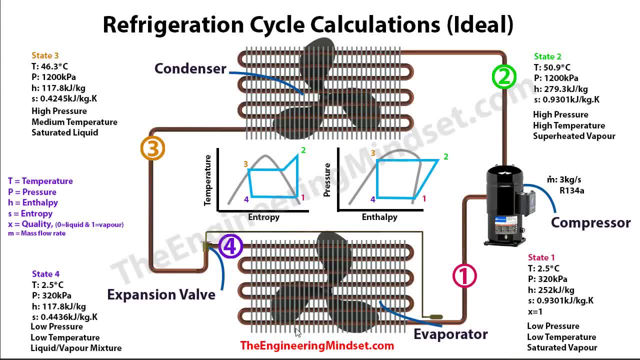 the temperature of the air coming off the coil. so the air on the- in this case the evaporator and the condenser- are both fan based. so if you want to know what the temperature of the air coming off of this is going to be, then you can have a.